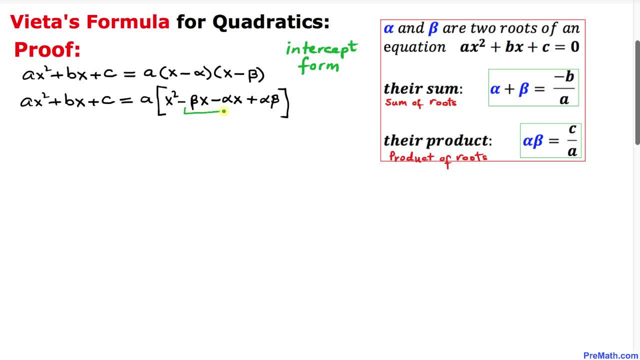 and now we can see that there is x in common between these two terms. So therefore, I have brought this x outside as a factor. so, inside the parentheses, we got alpha plus beta, x minus alpha, x plus alpha times beta, and now we can see that there is x in common. 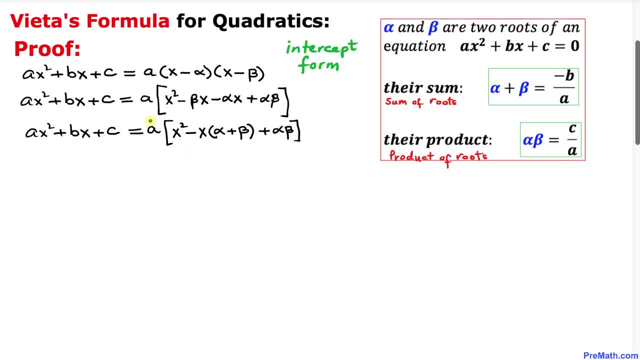 between these two terms. So then, this formula is again the same, but it can be written as ox square minus b over a plus beta, plus beta. The rest is same. And now, in this next step, let me go ahead and distribute this a along with these terms, So this could be simply decorate in as a x square minus a times. 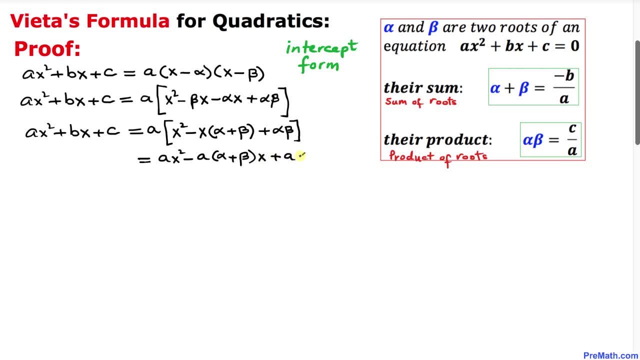 alpha plus beta times, x plus a times. let's go ahead and compare the coefficients. let's look at this thing on the left hand side minus bx, and in this right hand side we got the coefficient of x over. here we're going to equate them. so 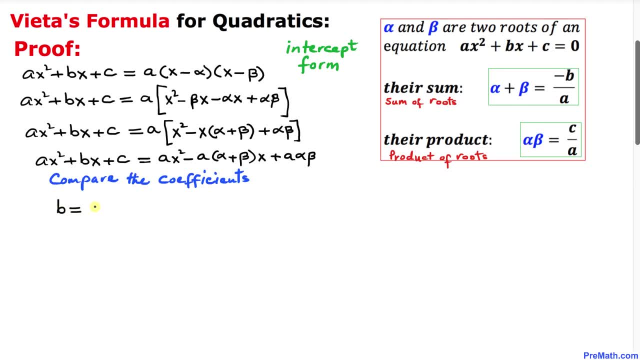 therefore, i can write b equal to negative a times alpha plus beta. now we are going to equate the constant term c on the left hand side and, on the right hand side, a times alpha beta. therefore, i can write this one as c equal to a times alpha times beta. let's go ahead and divide this one. 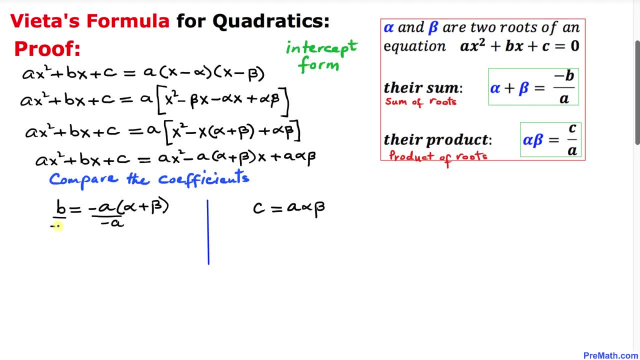 by negative a on both sides. so therefore our alpha plus beta is equal to minus b over a. and likewise, here i am going to divide both sides by a, so we are going to get alpha times beta equal to c over a. thus we got alpha plus beta. the sum of these two roots turns out to be: 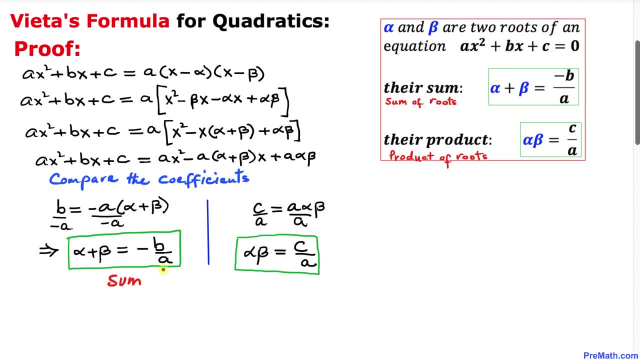 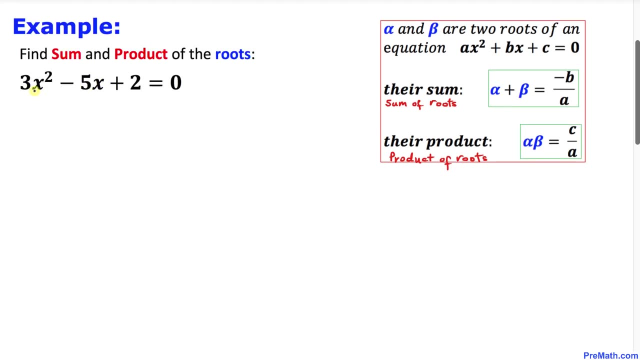 negative b over a. so these are our sum of two roots, and here alpha times beta equal to c over a, and that is the product of the over a of our these two roots, and that's our proof. and now let me show you an example we are looking at.